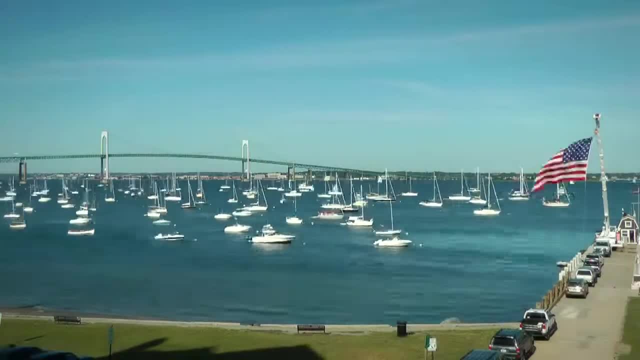 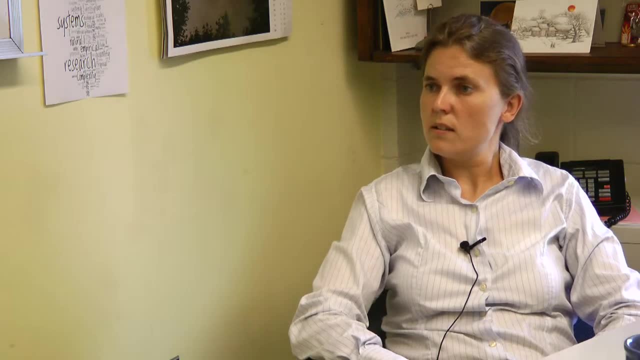 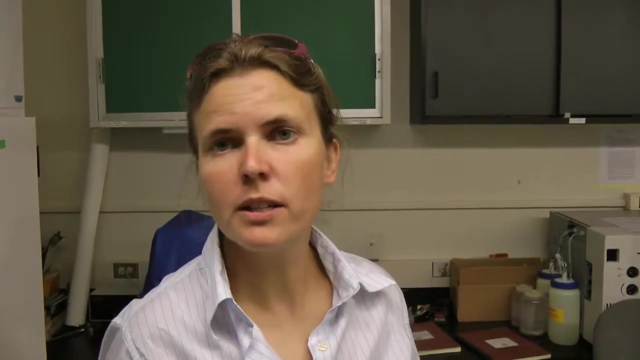 the tides are moving the water along, There's always fluid moving around, there's always an infection. Nothing stays the same for very much time, So a lot of our studies happen in the lab, So this room is really noisy. This is our life lab, where we culture organisms, maintain them. 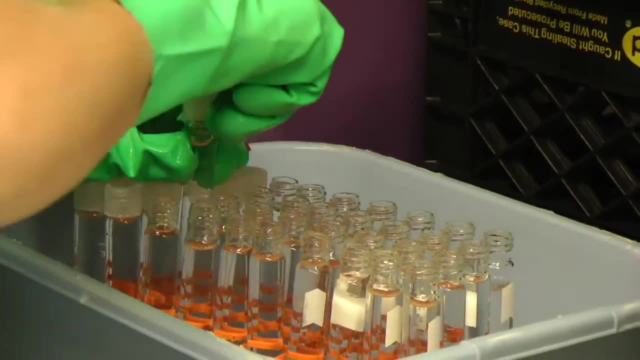 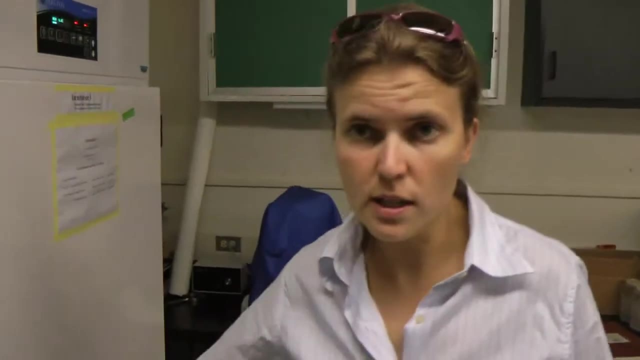 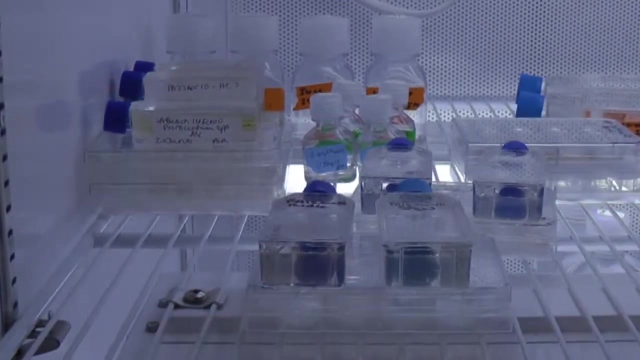 and we call it the life lab, because anything toxic is strictly forbidden. So any soap, any preservatives, anything that can kill these really sensitive organisms, And I'll show you how we keep them. There's dozens of different types in here. When we bring these organisms into culture, we have to figure out a whole bunch of things. 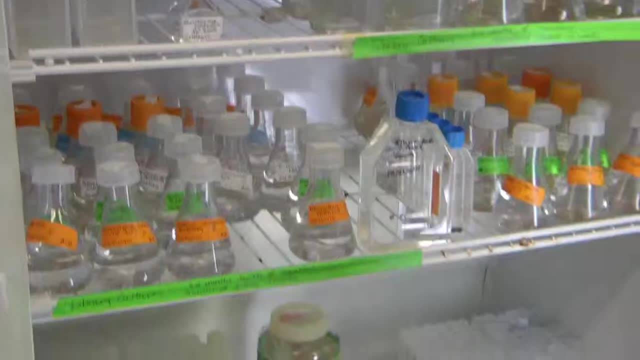 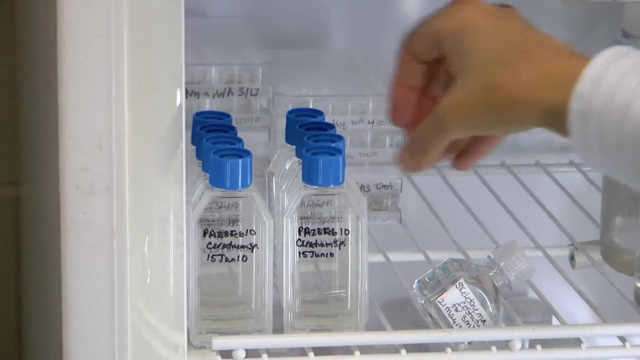 What are the conditions they like? What are the light levels, What are the temperature levels? What kind of food do they like? And most of the organisms do not do well on culture, So most of the plankton from the ocean are very difficult to maintain. 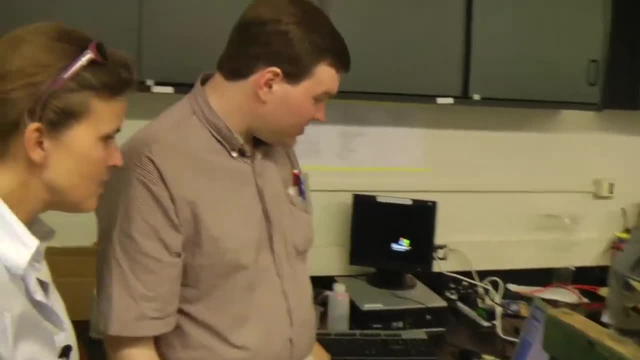 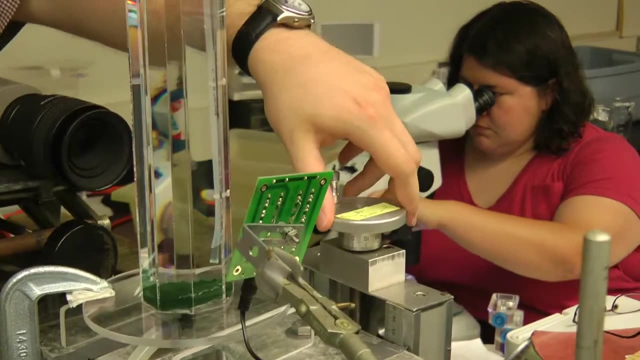 So what are you doing there right now? Are you seeing anything? I actually have seen quite a few. What did you put in there? Some acacia sanguinea? What Henry's done here is he's set up a water column that's stabilized. 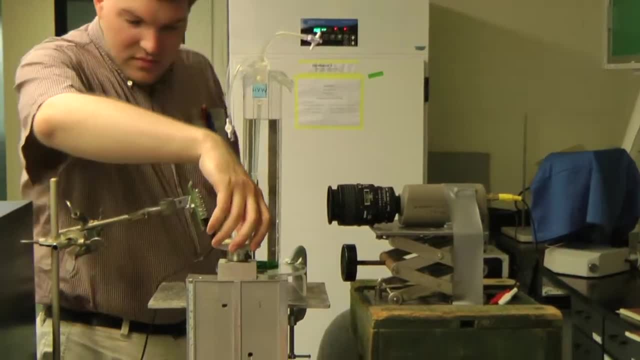 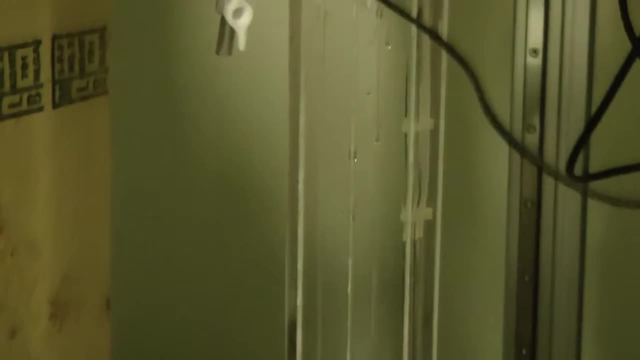 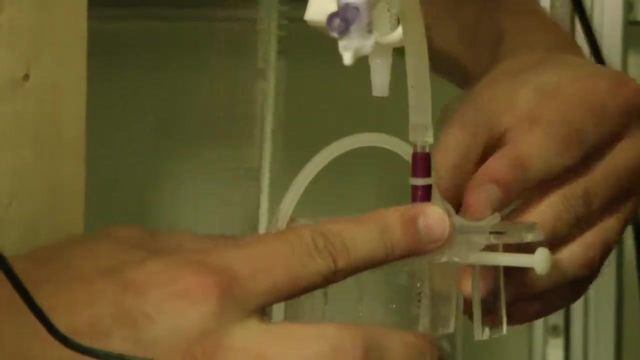 and then, through this tubing, he can introduce different kinds of organisms and, with this camera, observe them. These columns allow us to have an environment that's stable over time and observe these organisms in as natural an environment as we can. It may be a day or two days. 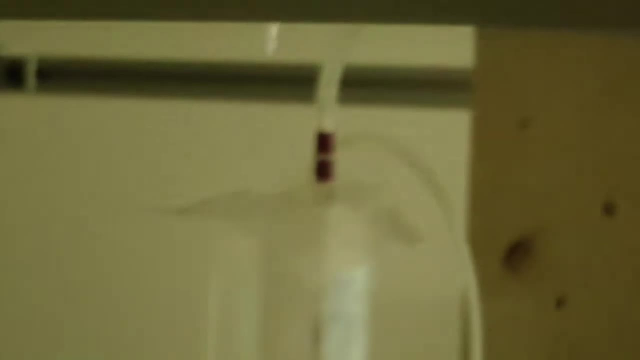 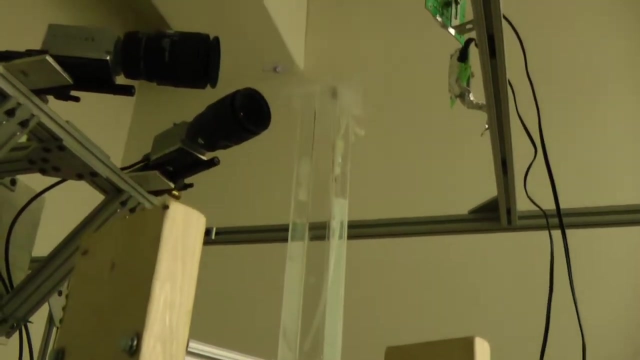 And remember, these organisms divide on the order of once a day, so a day is their lifetime, So we're seeing them for a really long time. These videos are then analyzed with respect to the abundance and distribution of the organisms, but also their movement behaviors. 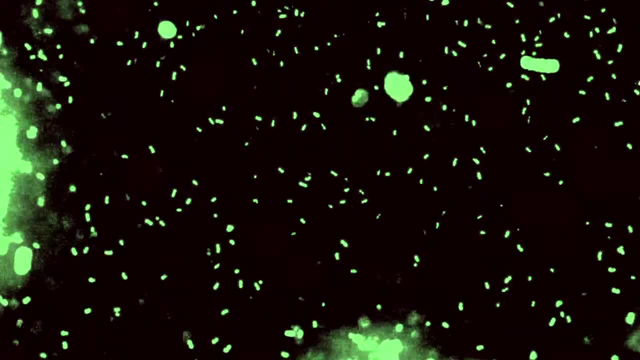 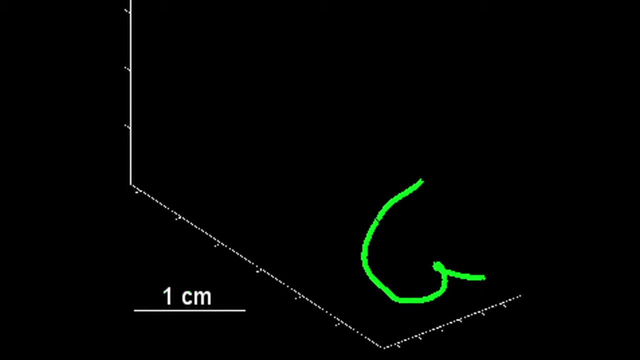 We're really interested in how organisms move. We've observed that some phytoplankton literally avoid their microzoo plankton or heterotrophic predators. That is a complexity in interactions that, to my knowledge, hasn't been observed before.